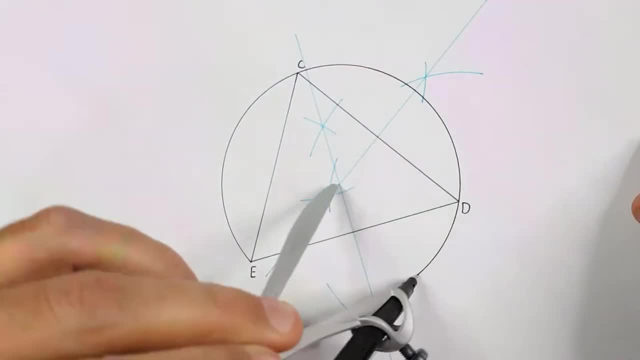 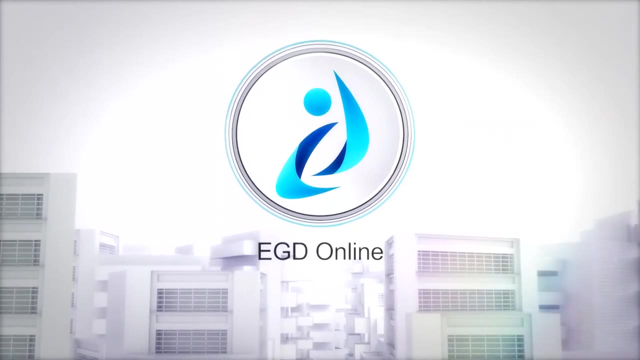 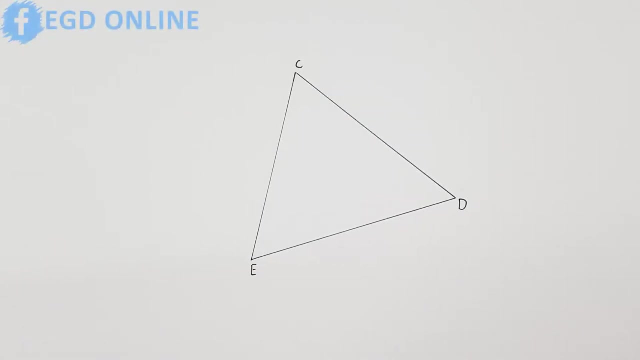 In this video, I'll show you how to construct a circumscribed circle. Hi everyone, and welcome to another video from EGD online. In this video, I will show you how to construct a circumscribed circle And, as always, I use a blue pen to show my construction lines. 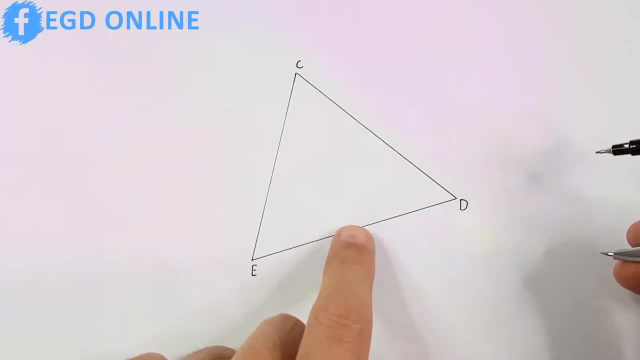 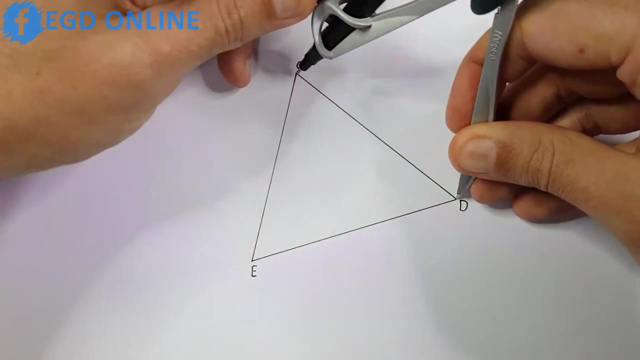 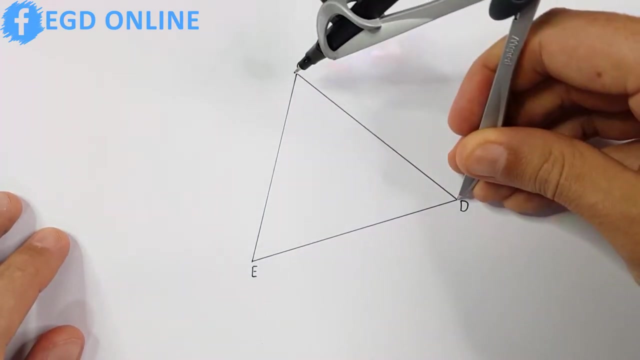 For this method you will require your compass. You are going to have to divide two of your three sides of your triangle using the middle point method. Using the full length of the side to apply the middle point method might use a lot of space. 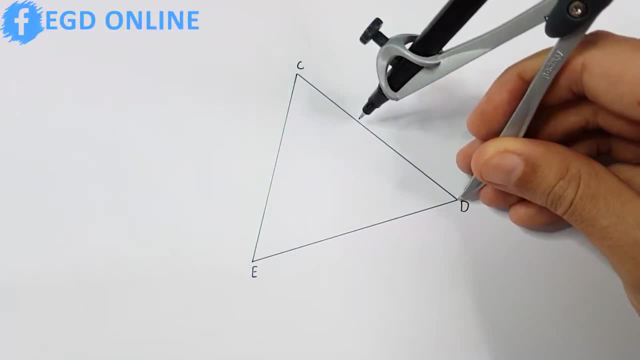 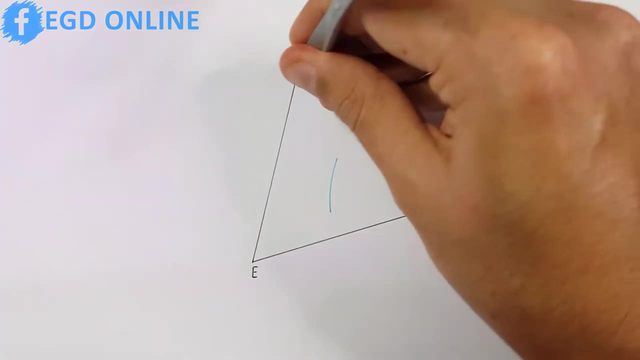 So, instead of doing that, adjust your compass just to more than half the length of the side. If you don't know how to apply this method, please comment below. Please go have a look at one of my previous videos where I show you how to apply the middle point method. 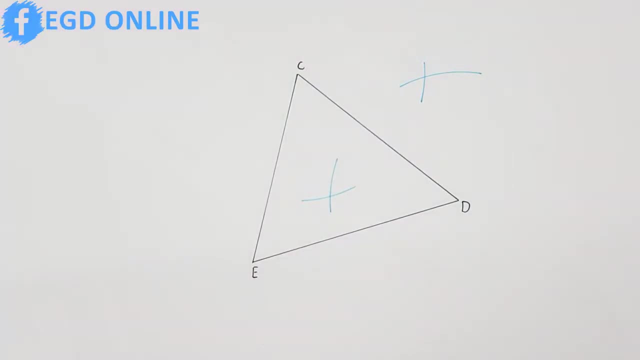 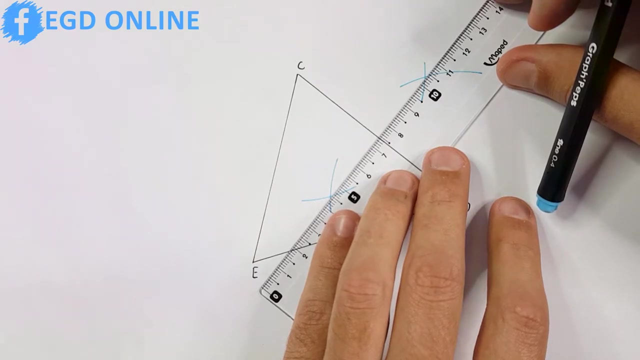 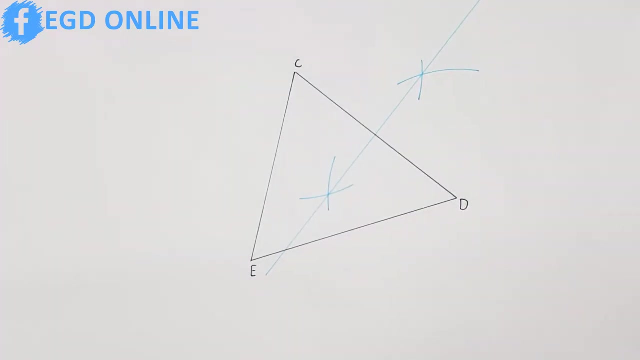 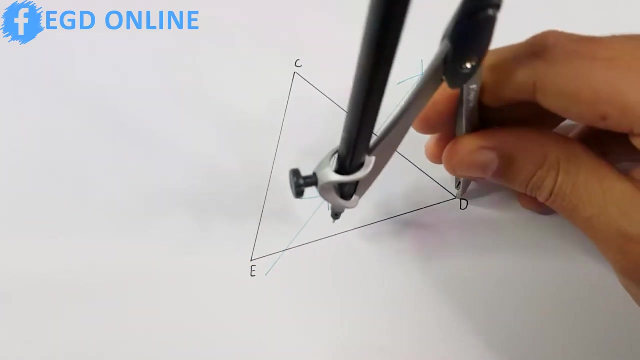 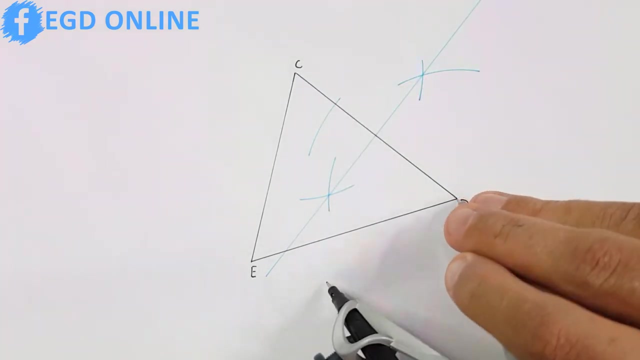 The link to that will be in the description. Next I will apply the same steps to side ED. The middle point method is to start from the middle point of the side. You need to go through the middle point, then you have to go through the middle point. 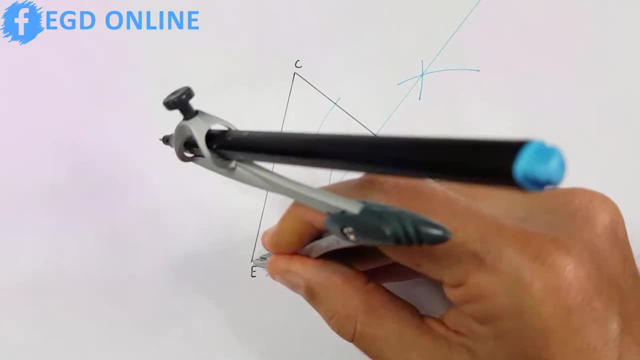 and take your time. Subtract the first point you want to go to or the middle point of the side. Add the second point to the middle point. Add the first point to the middle point And then, after you are done at this point, 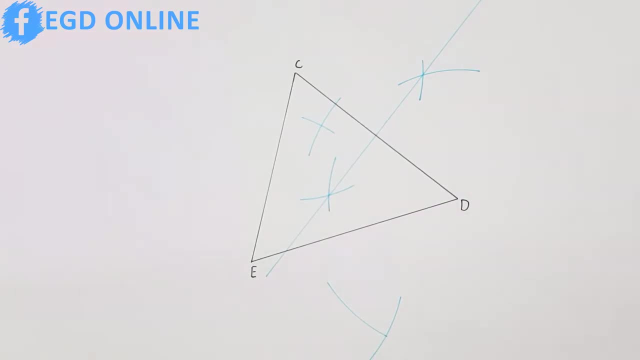 you can add the next point over here. So I'm just going to add this point over here. I will go over here till the end of the video and you can see the difference. But first let's get back to our basic construction. 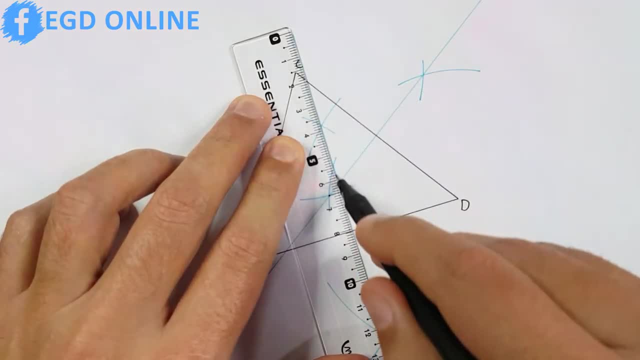 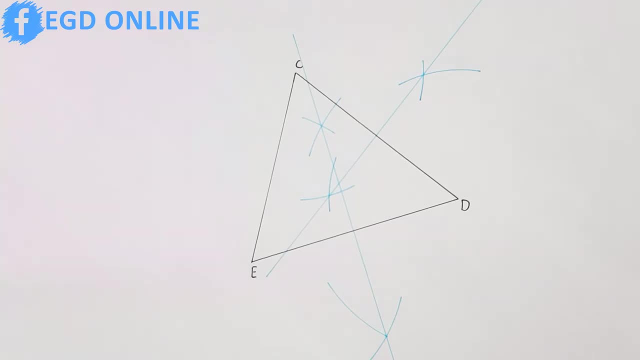 I'm going to go back to the beginning point. I am going to go double check the way I approached the center point. after applying the middle point method on two of your sides, the middle point of your circle will be determined where these methods section each other.